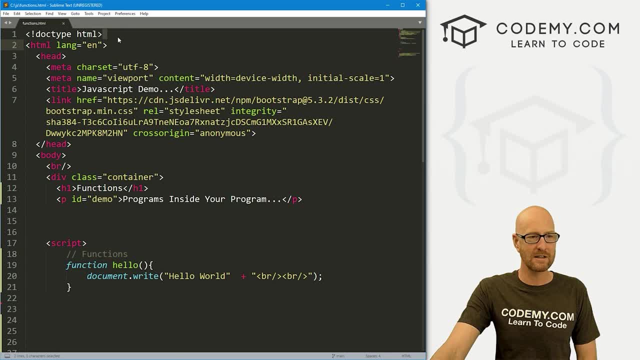 HTML. in this case we have something called program flow. we start at the top here And the interpreter- or whatever the web browser in this case- reads the first line, then it reads the second line, the third line, and it just keeps going down And it executes everything it sees. 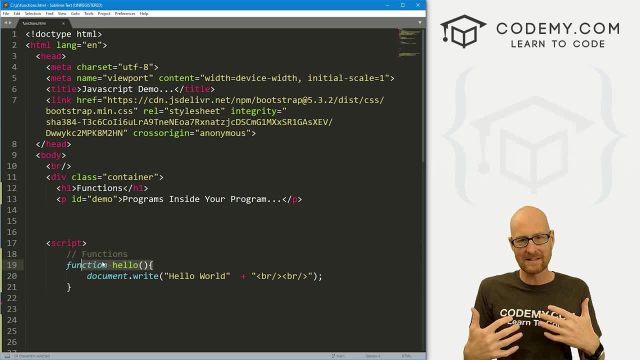 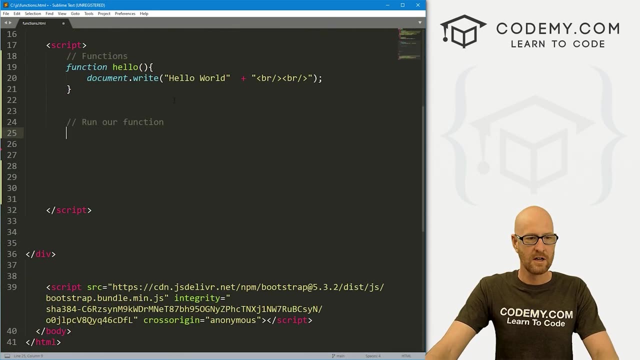 Here with a function. it sees it, it reads it, it understands that it's there, but it doesn't execute it because it's a function and functions only get executed when you call them. So how do we execute, How do we run a function? Well, let's go run our function here. Bring this down to run any. 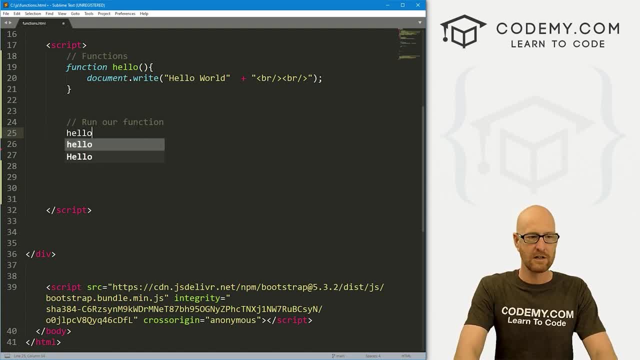 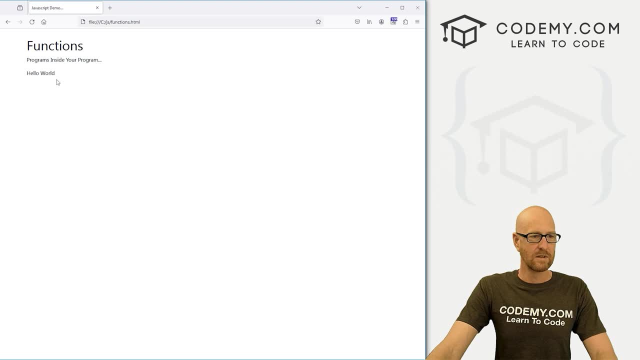 sort of function, And this is true in basically all programming languages. you just call the function And we use our parentheses here. So now, if we save this and run it, we see Hello world gets printed onto the screen. Very cool. Now, right here I've just sort of document written. 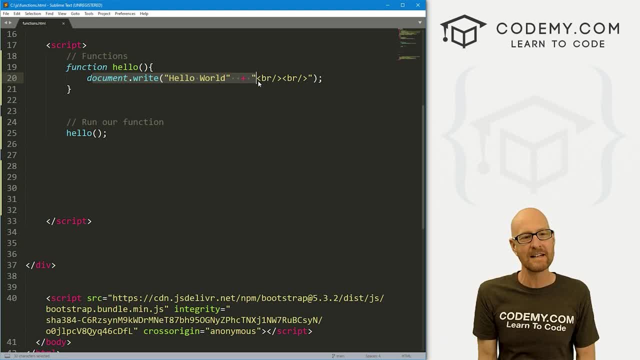 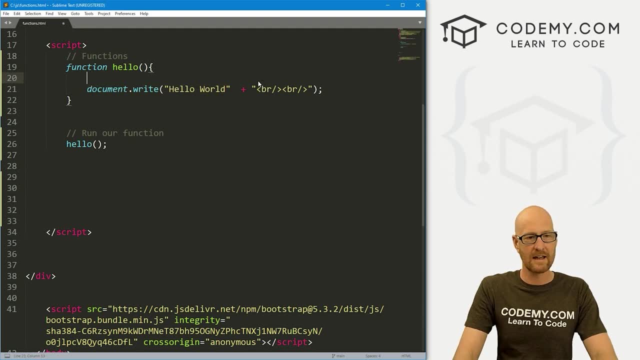 out in our function And normally I mean you could do that. obviously we just did. That's not really what you want to do with a function. Usually with a function you want to return something, right. So let's say: what do we want to return? we want to return whatever is in here. 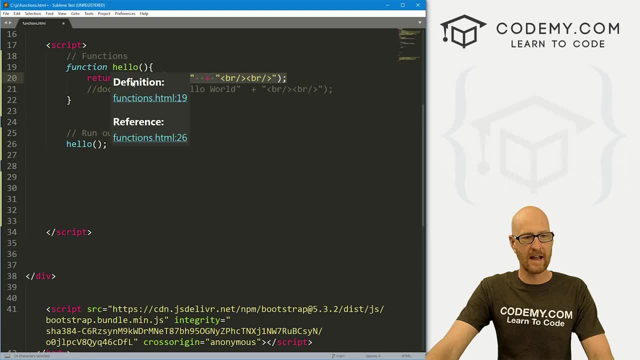 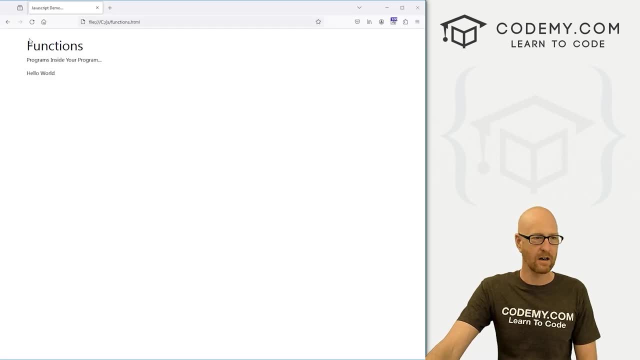 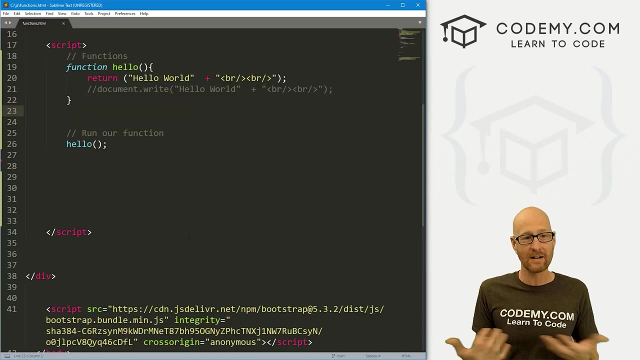 So let's comment this out. This function gets run and it returns this whatever's in here, right? Well, if we save this and come back over here and hit reload, we're not going to get anything. Why is that? Well, because this is sort of important. we returned it, but we didn't do anything with it. 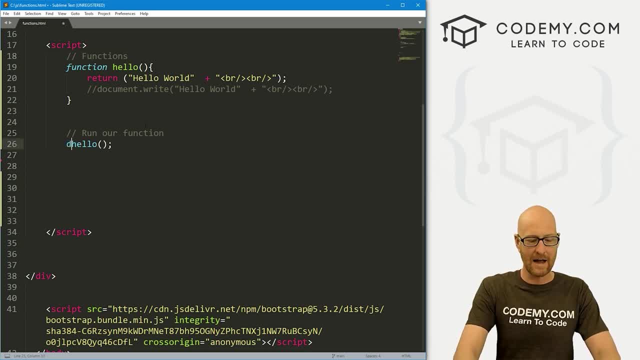 right. So if we wanted to actually print it onto the screen, we would have to document write it out. So let's go document dot write and then put all of this. whatever you know, whatever gets returned from running this function, we'll just get you know document written out on the screen Now. 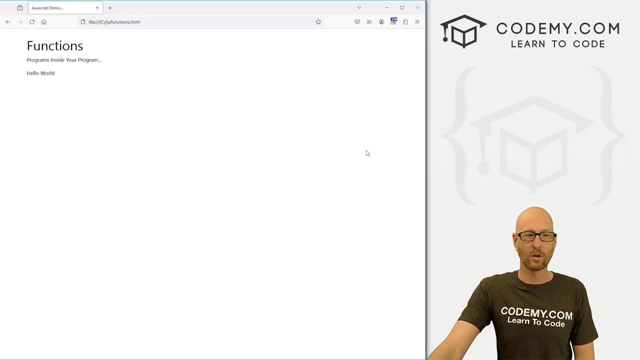 in this case, if we save this and run it, we're going to get what we expect, Hello world. So sort of keep that in mind, you can do that. But if we save this and run it, we're going to get what we. expect Hello world, So sort of keep that in mind, you can do that. But if we save this and run it, we're going to get what we expect Hello world, So sort of keep that in mind, you can do that. But if we save this, 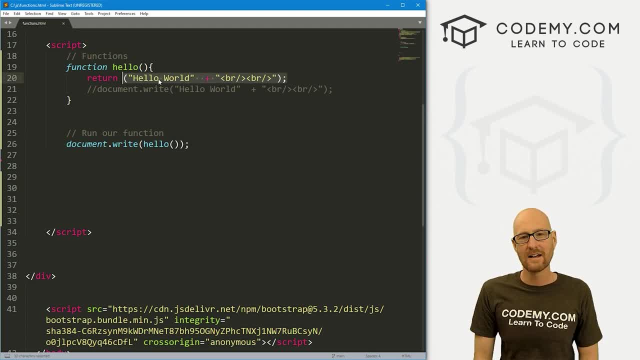 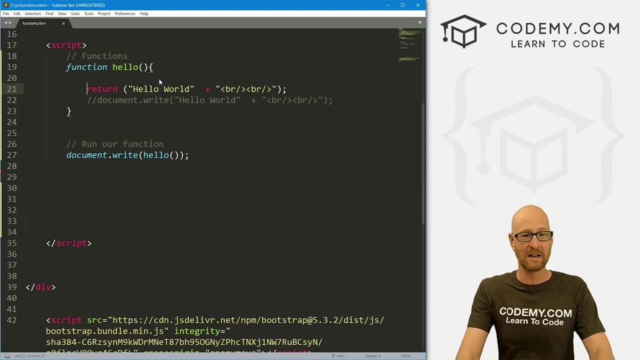 either way, it's sort of more best practice to just return, because a function is usually going to do a lot of stuff, a lot of things. right, Because a function is usually going to do many things. we've just done one thing here, one little line of code, but your function could have hundreds of. 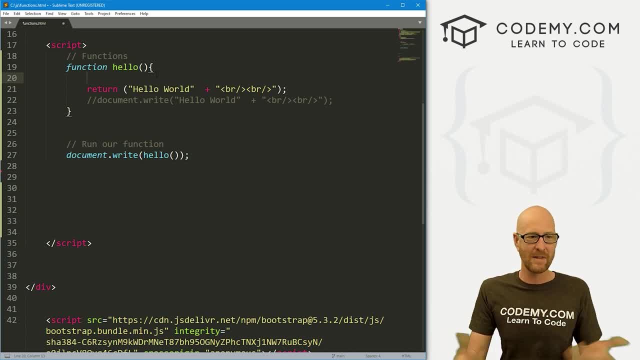 lines of codes, dozens of lines, 1000s of lines, right, And then when it does all that stuff, it's going to return something at the end of all that. And then you're, you know you're going to. 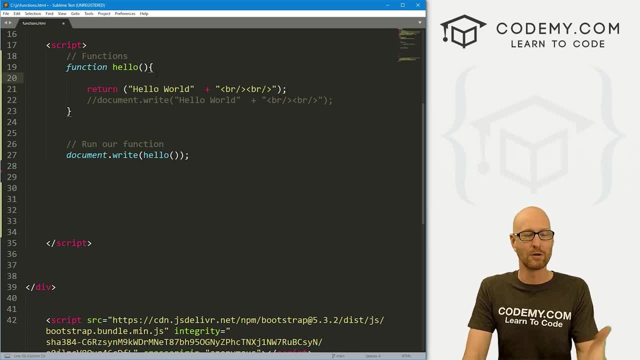 return something like we've done here. So it's sort of you know, best practice to return from a function. you don't have to, like we just saw, But that's the best thing to do. So, okay, that's cool. What else can we do with this? Well, we can pass stuff in to our function. 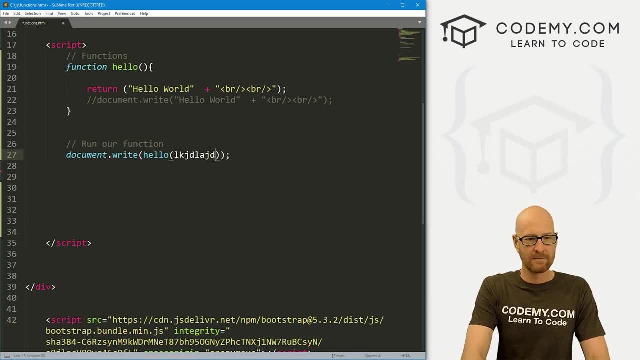 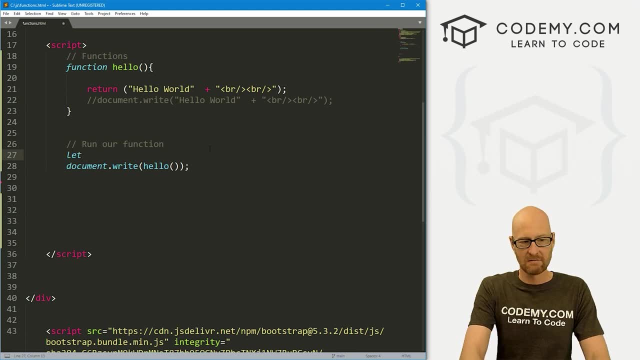 by passing it in right here, right. So I should mention we're document, writing this out to the screen. there's many different ways you could do this. you could say: let something equal Hello, like that, And then you can come down here and print out something right, create. 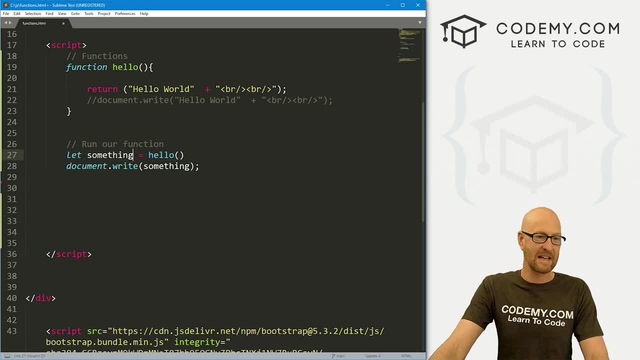 a variable, assign whatever gets returned from this function into the variable and then use that variable to do something later on. That's usually what you're going to do- something like that. I don't want to make this that complicated, So we're just going to keep it. 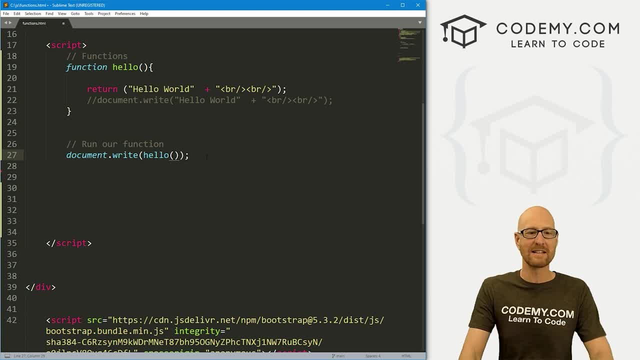 like this. So back to passing things into a function. Like I said, we can pass things into a function. let's say we wanted to pass a name So I could type in quotation marks and john, So the structure of this stays the same. I kind of just print this onto the screen. 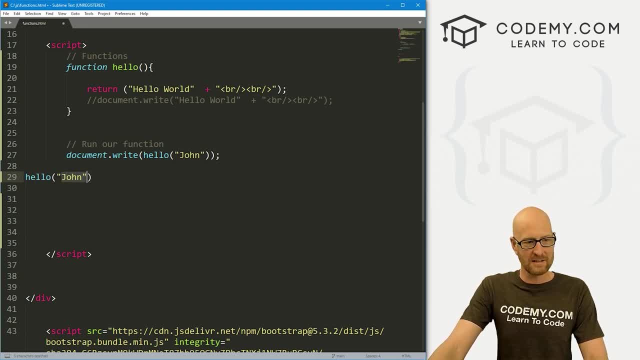 we're calling our function, we've got our parentheses. Inside the parentheses we're passing some attributes, some thing, right. So now we have to change our function around. we need to account for information getting passed to our function, And we do that right here. So let's create a variable And let's call. 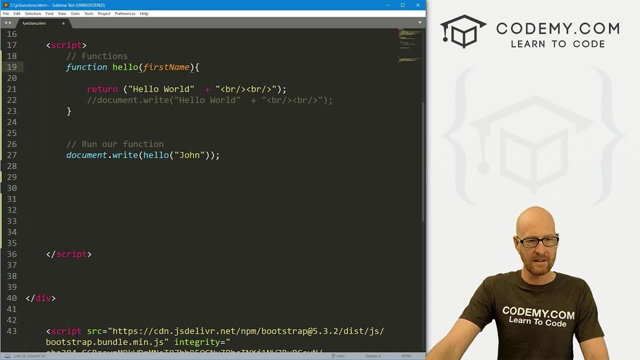 this? I don't know. let's call it first name. Now this variable is going to be local to just this function. Like I couldn't come out here And you know, document dot, write First name, right, This would not work. 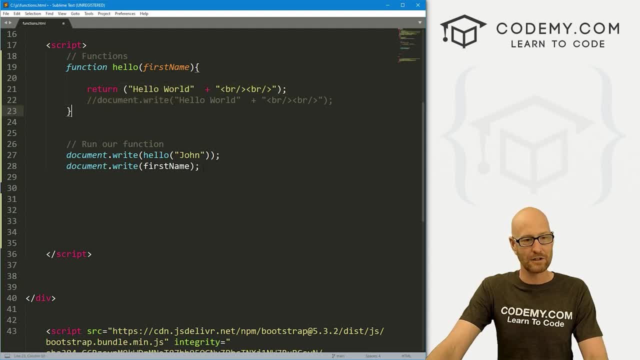 Because this variable can only be used inside of this function, right? So sort of keep that in mind. But now inside this function we can use this variable. So let's come down here And let's say: instead of Hello world, let's say plus, and then print out first name. 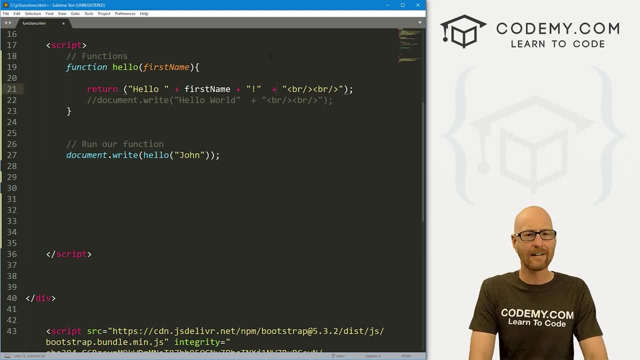 and then maybe another plus and let's give an exclamation point because heck, yeah, this is exciting. So now we've got first name, we're passing this in. Now we can use this however we want inside this function. So if we save this, come back over here. we're going. 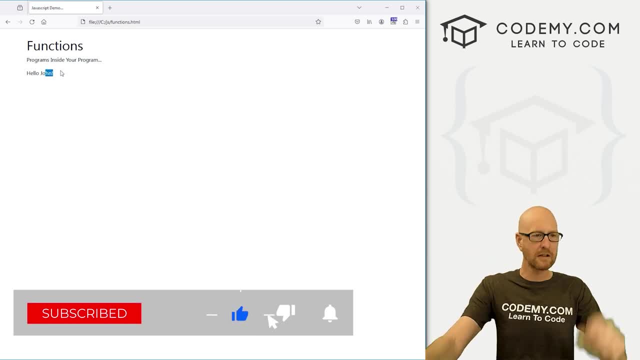 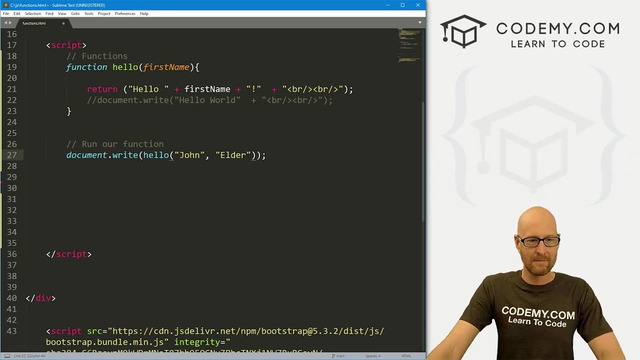 over here here reload. it would be as you would expect. Hello, john, whoo, exclamation point. There we go, So we can pass more than one thing here. we could say, john and elder, right, But again up here, we have to account for that. Let's say we don't account for that. 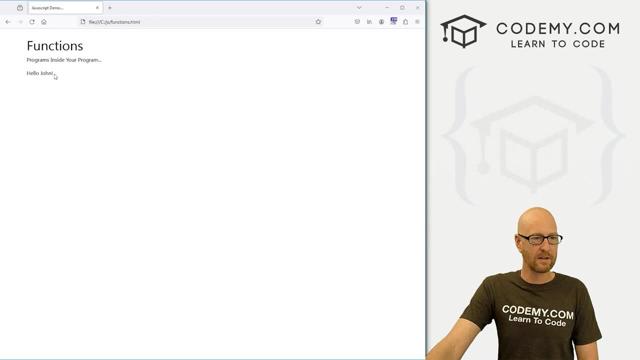 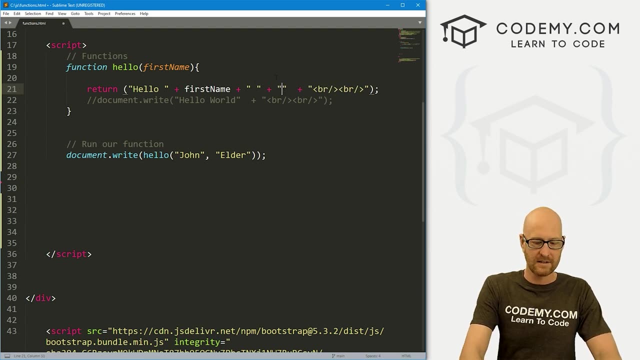 Let's just save this. we're gonna get an error here. So if we hit reload, well, now it still says john. But if we came down here and went like this and then say last name, we don't want. 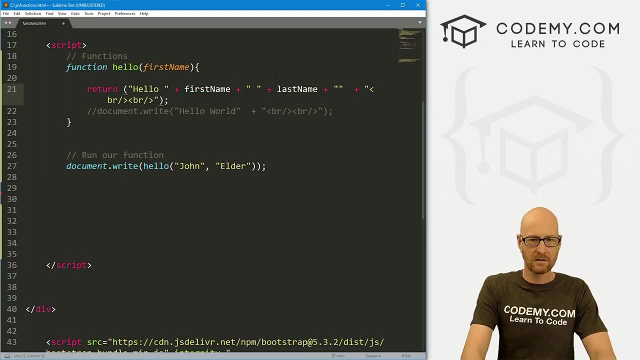 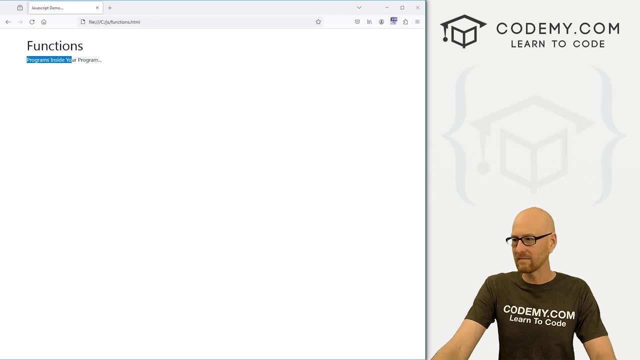 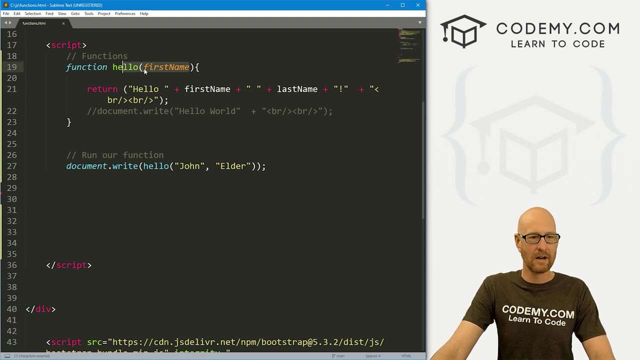 Okay, So we're gonna hit reload. we're gonna get just nothing. Suppose there's no error, but it's just nothing Because we haven't accounted for it up here. We're passing two things, But we've only got one thing in our function here, So we have to create another variable. 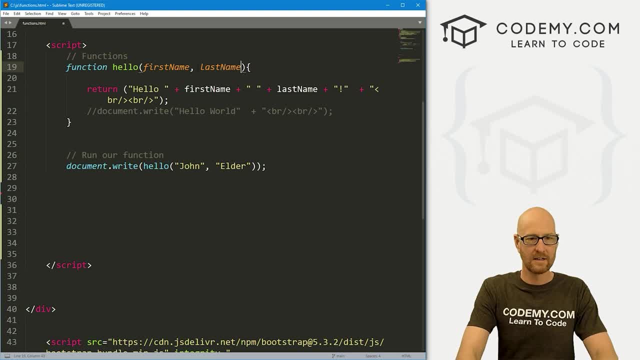 So we'll call this last name, Right? So there are two items here that we're passing And now we have two variables. The first thing listed here is going to be the first variable listed here. The second thing listed here is going to be the second variable. JavaScript knows to match these up. 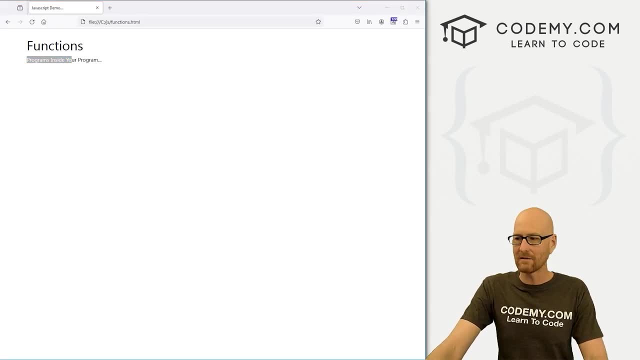 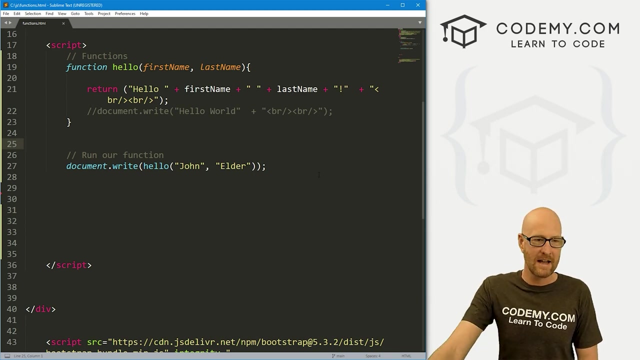 right. So all right, go ahead and save this and run it And it's gonna say: hello, john elder exclamation point. There we go. So those are functions- super easy, But just incredibly important. right, you're going to use functions for everything Now. one nice thing about this is: 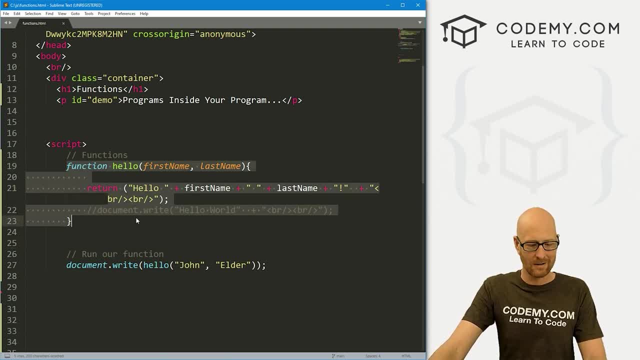 like we can take this code and put it anywhere, right? It's kind of weird to have a giant function right in the middle of your HTML page, Right? So we talked about way back at the beginning of this playlist. we can get rid of this And, for instance, come up here: 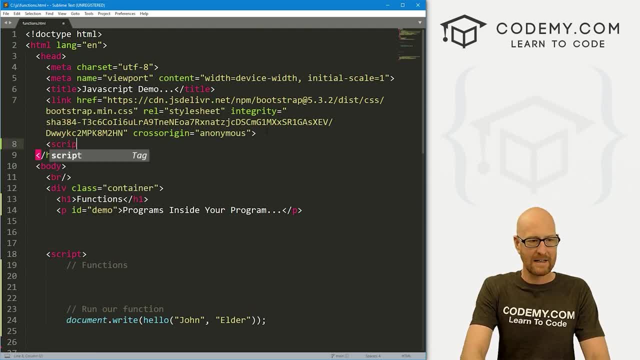 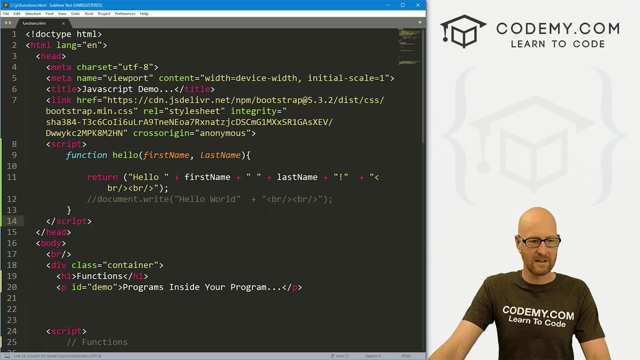 to our head tag And maybe we want to put this in our head tag So we can create a script tag and then close that script tag. If we save this, let's come down here and change this a little bit, just so we make sure let's call this Tim elder. 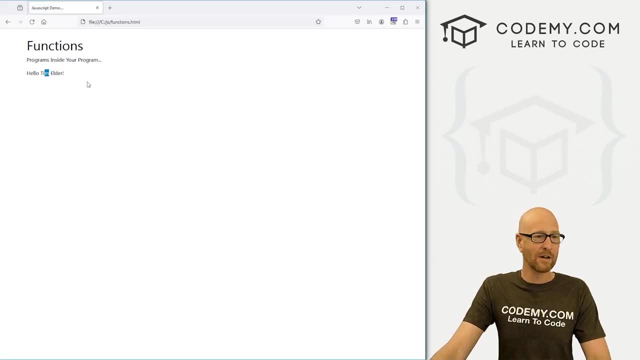 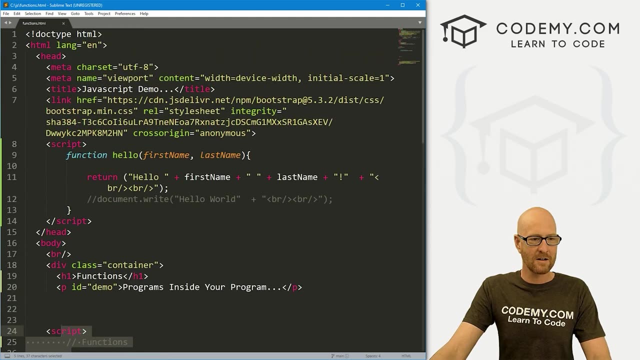 I don't know any Tim elders but I'm sure they're out there. Now, if we hit reload it says Tim elder. the program hasn't essentially changed at all, But we've moved all of that functional code way up here, sort of gotten it out of the way, And that's nice right. 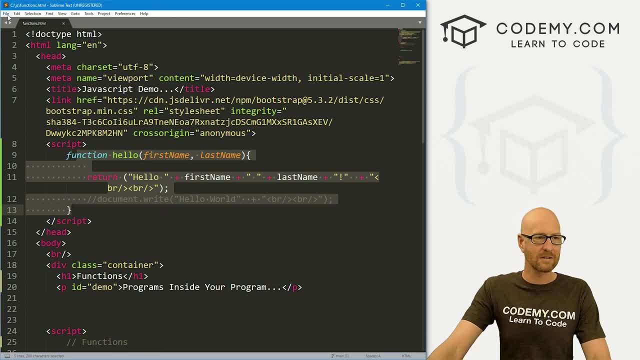 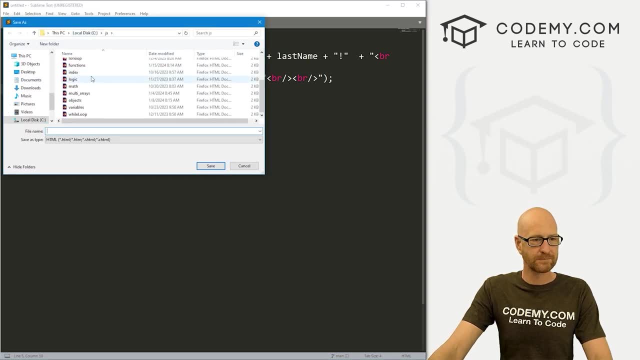 We could do that, But we could also create another file. So let's go file new And let's paste in that code And let's file save as an inside of our same directory. Let's call this my function: dot j s. 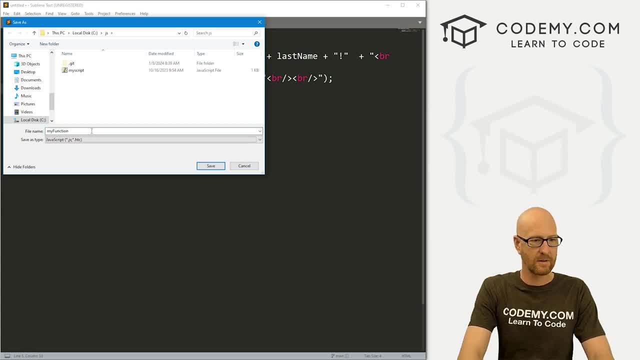 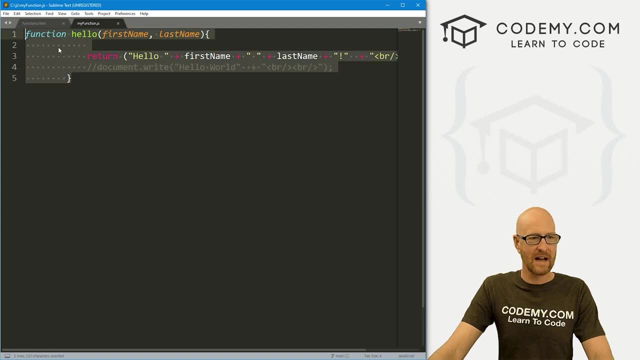 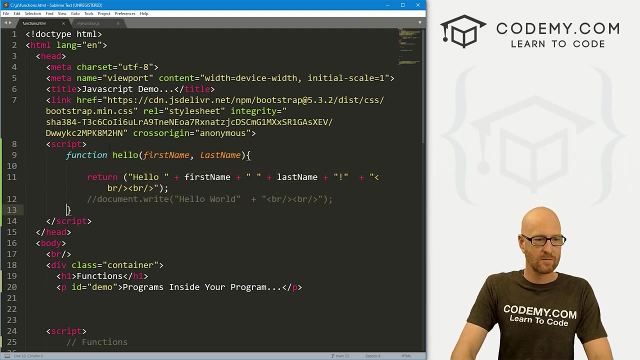 Change this to JavaScript. There we go. We already have a my script. Now we're going to call this my function, And if we save this now, we've got this code in a separate file, which is super useful. right Now we can come up here and, instead of printing all of this, 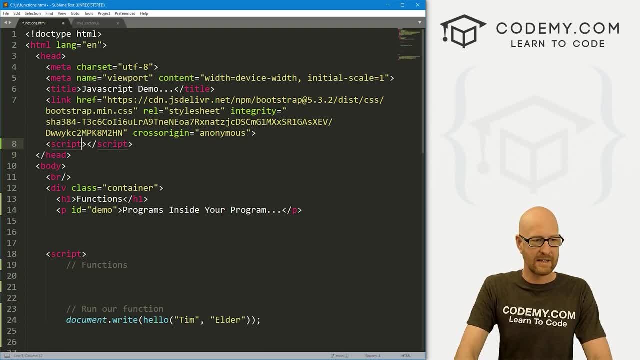 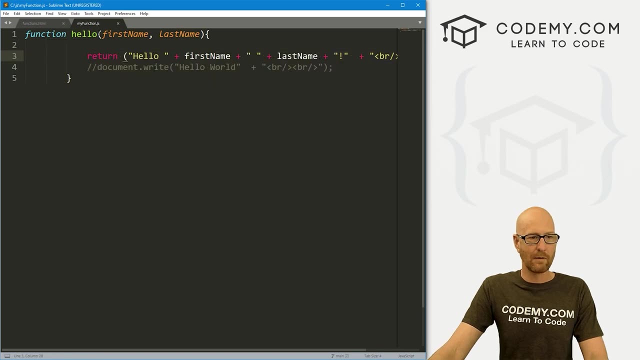 in our head, which is, you know, kind of sloppy. we can instead just give an SRC and pass in my function dot j s, And that should now load that script in the background, which is this thing right here, And then, when we want to call it, it will return this. of course, it returns it down. 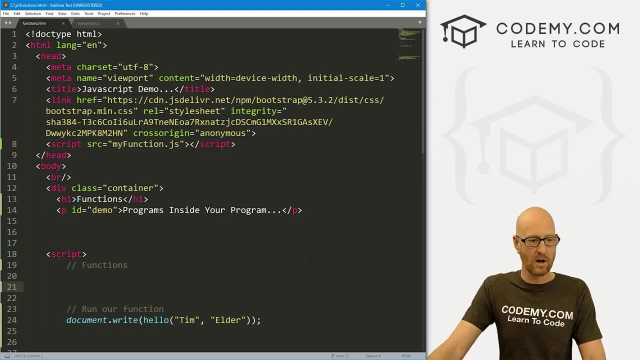 here And then we can print it out onto the screen wherever we want to print it out onto the screen. So if we save this, come back over here and hit reload- nothing has changed. Let's go ahead and change this back to john elder, just to make sure this is running and 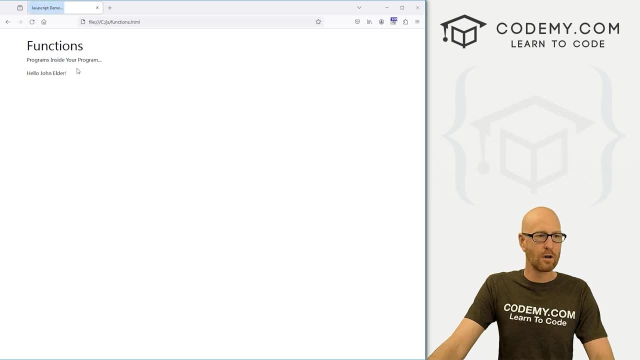 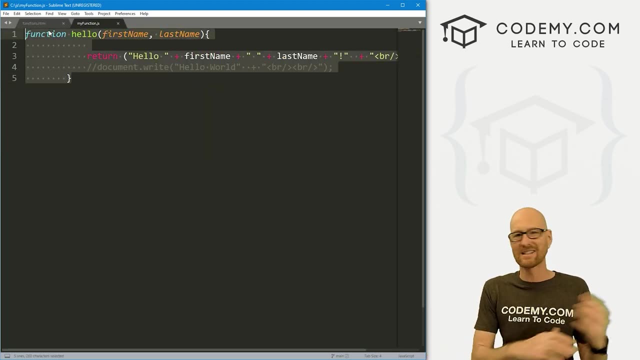 working. So we make a little change. john elder, boom. hello, john elder, And that is awesome. So a lot of times you're going to do something like this: you're going to put all your functional code in some other file, get it off the web page, get it off the website and then call. 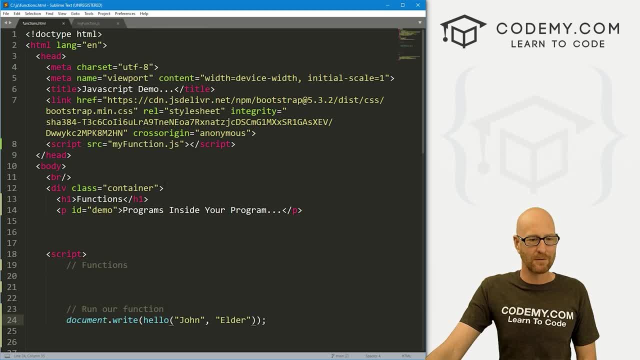 it from your web page. It's just better for program flow. it's better for readability. You know, this is obviously much less code on your HTML page, which is always a good thing And a very, very cool, So I'm gonna come back down here and paste this back in. 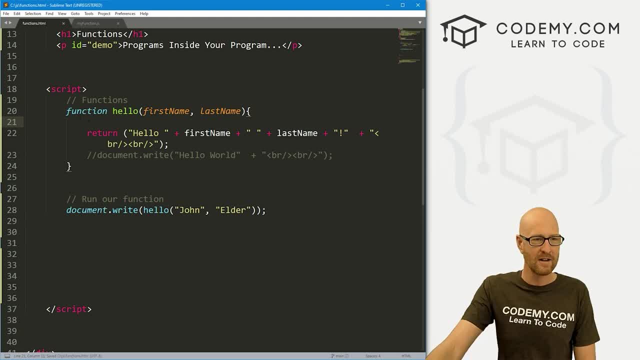 just so that's in the code, if you want to check the GitHub repository later on. But again, just remember, you're going to want to make sure that you're going to be able to do that, So I'm going to come back down here and paste this back in, just so that it's. 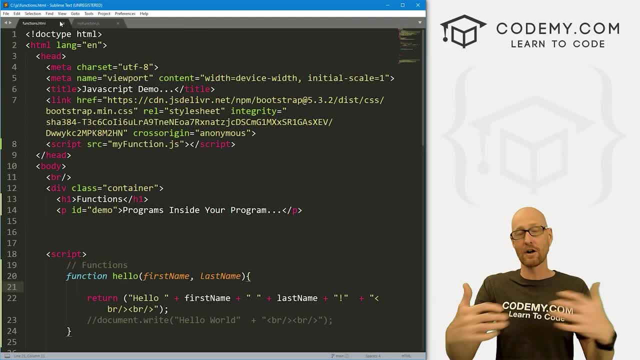 easy to remember, probably better to put your functions in their own file, especially if they're very complicated. If they're very complex, if you've got hundreds and hundreds of lines of code right, you're going to put that in another file And even here, like.